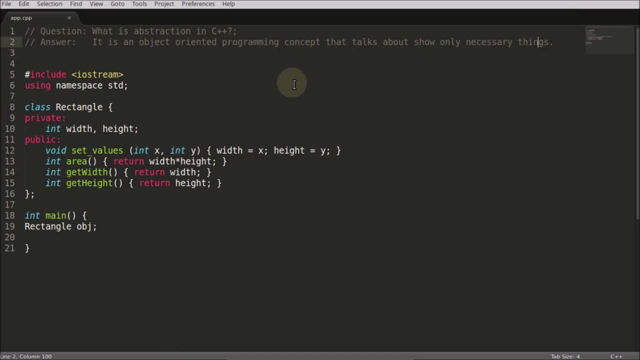 data hiding. Lots of people think that both are equal, but they are totally different thing, Okay. So first I will talk about data abstraction here. In next video I will talk about what is data hiding. Okay, so abstraction means you don't want to show how you have. 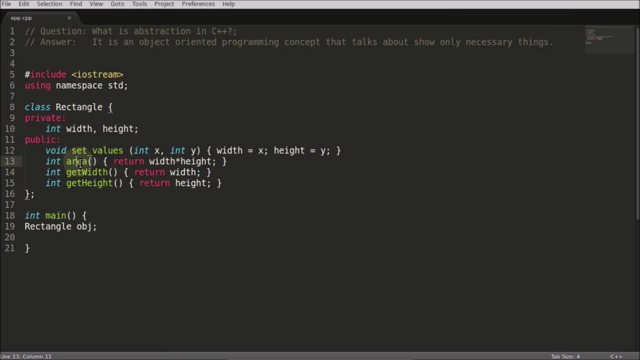 implemented something Okay, like some function. this is your function. you are calculating the area. you just don't want to show how you have calculated it. Okay, so I'll explain you in the layman language. Let's suppose you have some file which we call library. 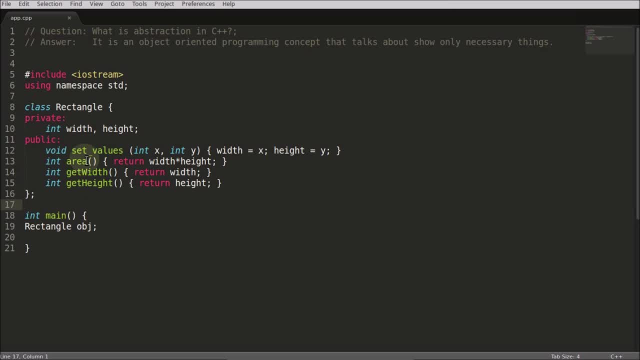 Inside that you can only see what are the functions like if this is the entity which is this class rectangle, And you can only see what are the possible operations available in this rectangle, like set values and get the area, get width and height. So these are the operations which 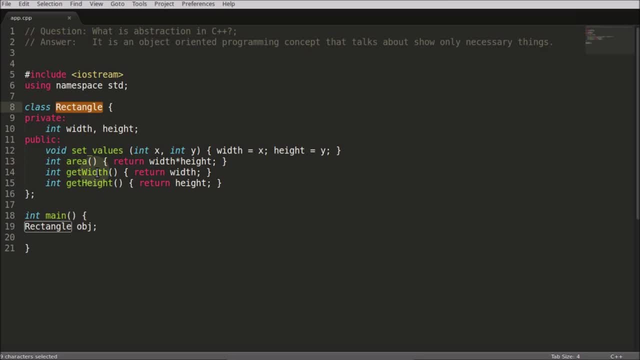 is possible on this rectangle entity. Okay, you will be able to see only this much. So that is data abstraction. you won't be able to see how something has implemented, like how the area is being calculated. This is very simple thing, So you might think that. 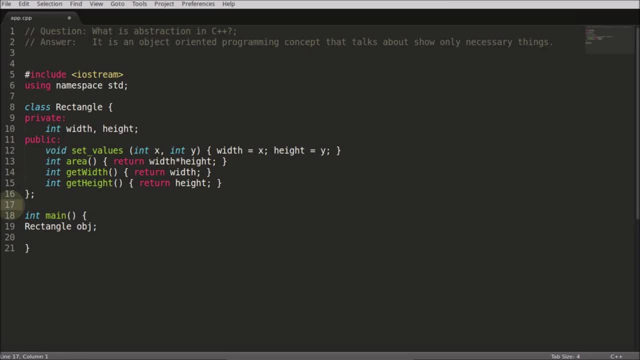 how to calculate the area. but let's suppose there is one expensive class, let's say rocket, And you don't want to share how the rocket flies. Okay. so there is one method: fly, Okay. And you have written very much complex code in that which you don't want to show to others. 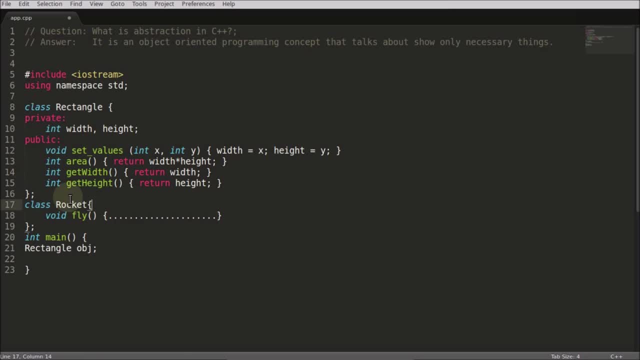 Okay. so what you will do, you will compile your code- I'm in this class- and convert that into a library And so that you are having this fly function. you just call the function and this rocket will start flying. Okay, you won't show what is happening inside that And user won't be. 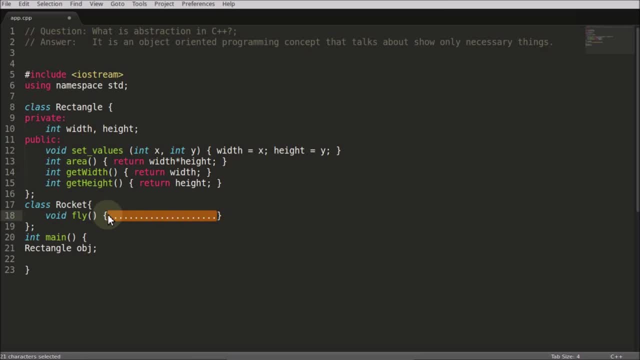 able to see that, And the reason could be anything why you don't want to show that. okay, So hiding the implementation part is called abstraction. Okay, remember this: you're hiding the implementation. Okay, you're not hiding the data. That is a different concept. I will. 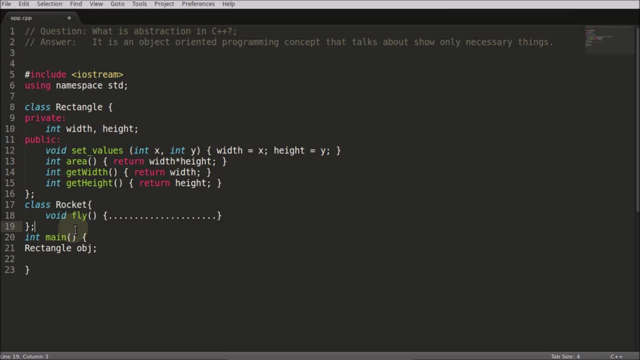 talk about that in my next video. Okay, So that's it. I'm done here. Thanks for watching and check out my other videos and prepare well, Thanks, Bye, bye.